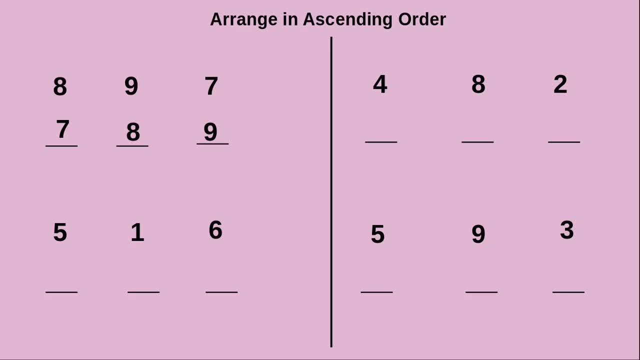 which number is remaining, 9.. So now we are arrange this number in ascending order. Next we will move back to another example. They given 5, 1, 6.. So, while comparing this number, which is the smallest number? Yes, 1 is the smallest number. First we are going to write the number 1.. After that, 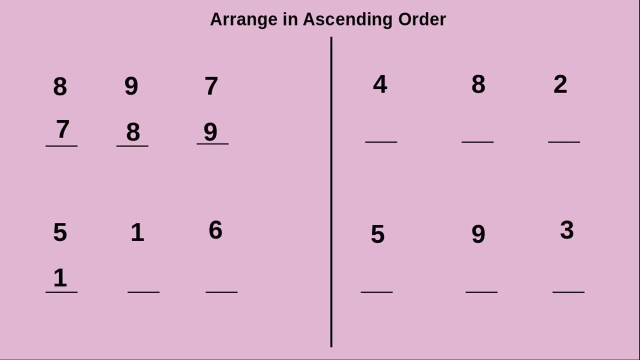 which is the smallest number? Yes, correct, 5 is the smallest number At last, which is 1? 6.. So now we are arrange this number in ascending order. Next they are given 4, 8, 2.. So which is the smallest number here? 2 is the smallest number. Next, what did we? 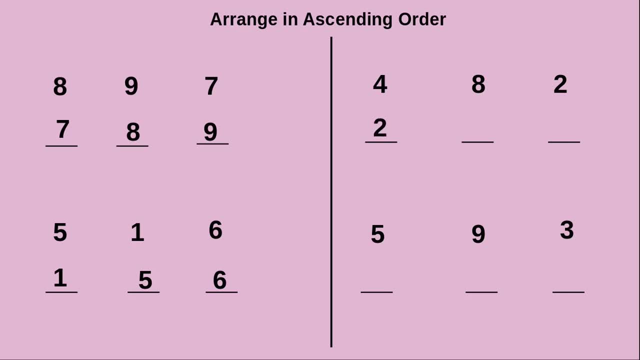 number. So first we are going to arrange the number 2.. After that, which one? 4.. So we are going to arrange 4.. At last, which number is remaining? It's 8.. So we are going to arrange number 8.. Now we will see the next example. They have given 5,, 9,, 3.. So which is the smallest? 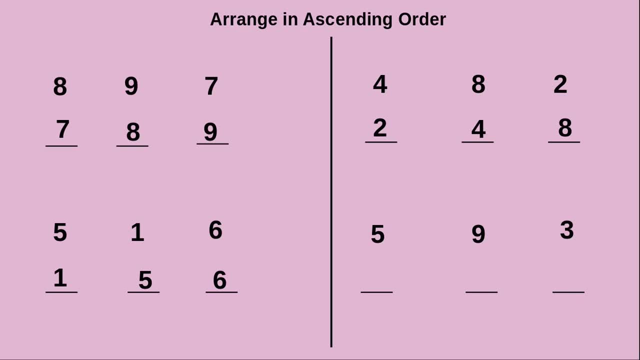 number here. Why we are going to see which number is smallest number? Because we are going to arrange this number in ascending order. So ascending order is nothing but arranging the numbers from smallest to greatest. So which number is smallest here? Yes, 3 is the smallest number. 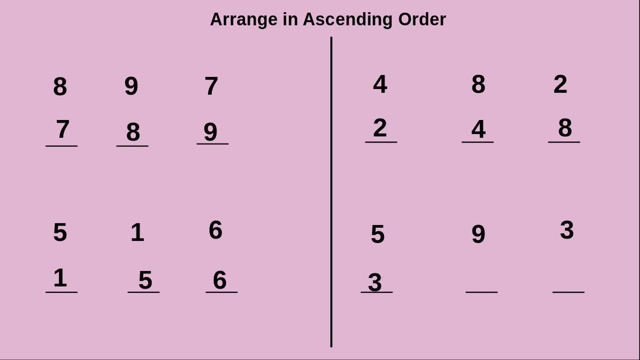 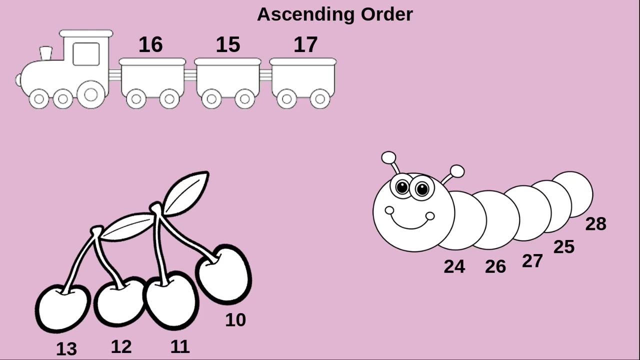 So we are going to arrange the number 3.. After that, which one is smallest? Yes, you are correct. 5. At last, which number is remaining? Yes, it's 9.. Now we will see the another examples. Here they have given 2 digit number. Now we are going to see how to arrange this number. So. 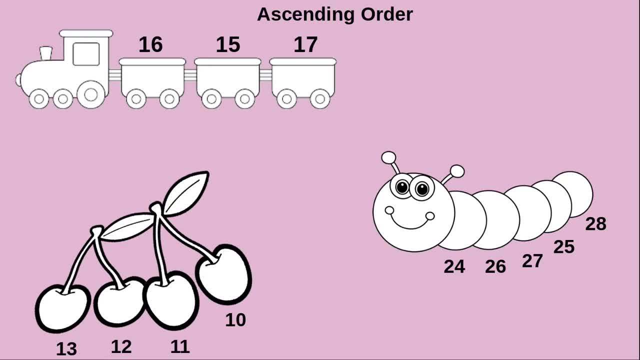 we are going to arrange this 2 digit number in ascending order. So first they have given some example, that is, 16,, 15,, 17.. Now we are going to arrange this number. So how we are going to arrange. First we want to see the last digit, that is 657.. Here, 657.. So which one is the smallest? 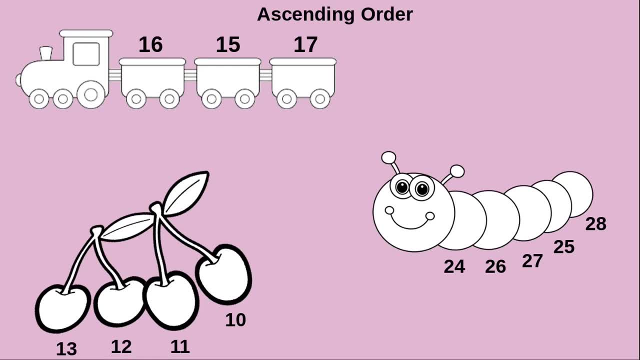 number 5 is the smallest number, So obviously 15 is the smallest number. So first one is 15.. We are going to arrange this number in ascending order. So 16 is the smallest number. At last, which one is remaining- 17.. So we are going to write 17 as it is. So now we are arrange this number in ascending. 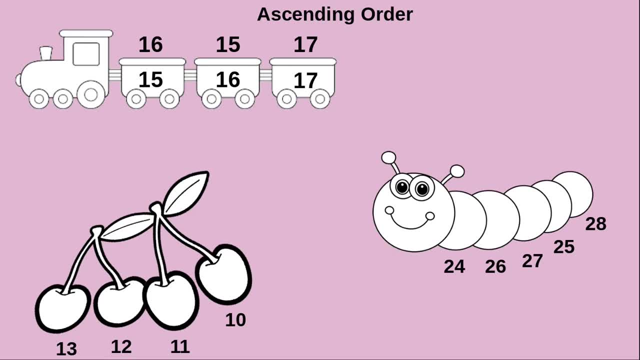 order. Next we- they have given 24,, 26,, 27,, 25, 28.. Now we are going to arrange this numbers. We know that. so ascending order is nothing but smallest number to greatest. So here which one is the. 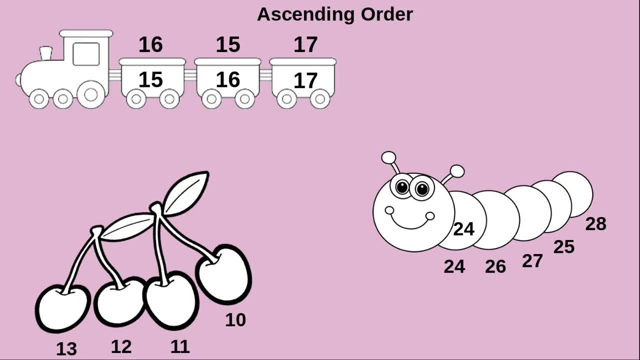 smallest number. Yes, 24 is the smallest number. So we are going to arrange this number in ascending order. First we are going to write that, After that which one, 25.. Next 26.. Next 27. At last, which is remaining 28.. So now we arrange this number. Now we will see the another example that 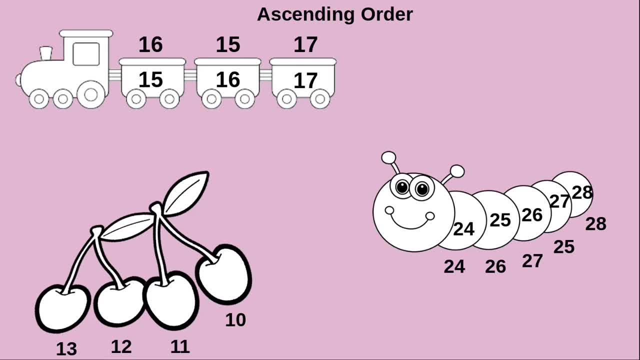 is 13,. 12, level 10.. So which is one? Yes, 10.. After that which one? 11.. After that, 12.. After that, 13.. So now we are arranged this number in ascending order. So now we all know what is ascending order. So ascending order. 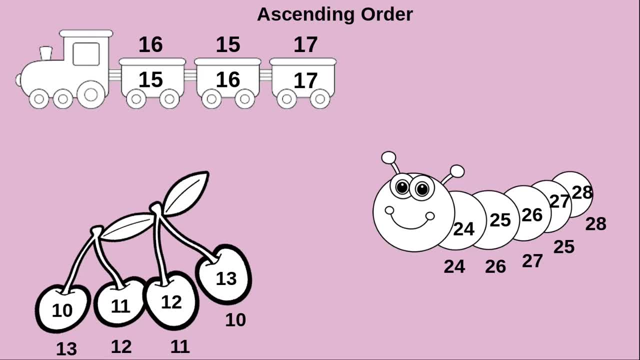 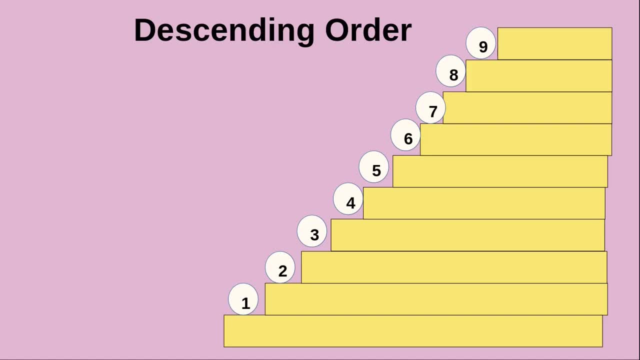 is nothing but arranging the numbers from smallest to greatest. Now, next, we will see descending orders. So what is descending order? We know that ascending order is nothing but smallest number to greatest number. So then, what is descending order? Yes, it is quite opposite. So arranging the 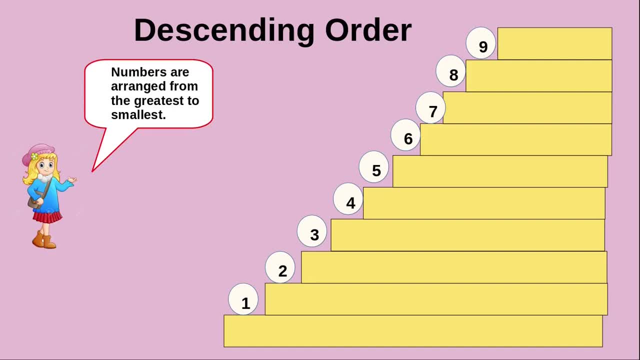 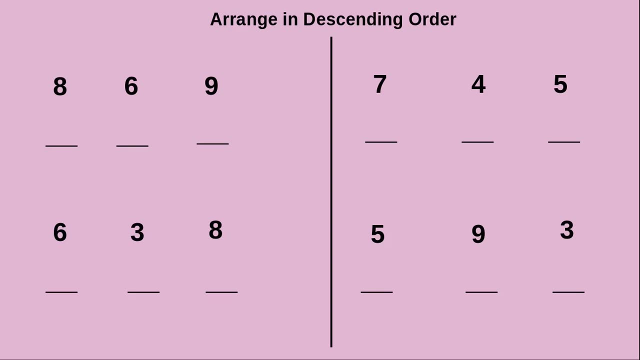 numbers from greatest to smallest. that is descending order. So we are going to arrange to arrange the number from 9 to 1 in descending order. okay, so descending order is nothing but arranging the numbers from greatest to smallest. now we will see some example how to arrange this. 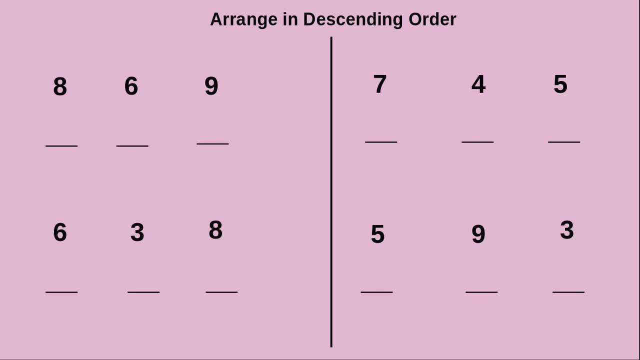 number in descending order. so first they have given 6, 8, 9, so now we are going to arrange this number in descending order. so we know that how we are going to arrange this number. so descending order is nothing but arranging the numbers from greatest to smallest. here which number is greatest? 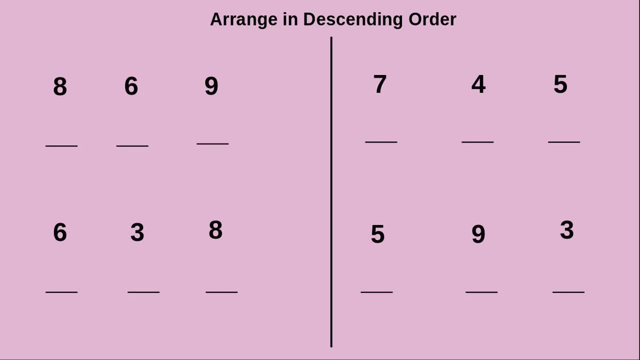 yes, 9 is the greatest number. so first we are going to place that 9, after that, which one is greatest? yes, it's 8. at last, which one is remaining? 6. so we are going to write as it is. so now we are arrange these numbers in descending order. next we will see the another example they have given. 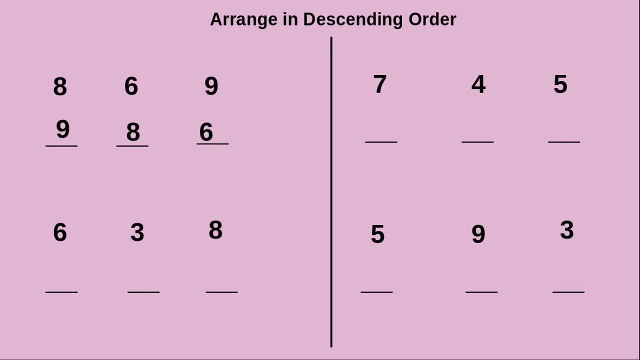 6, 3, 8. which one is the greatest number here? any guess? yes, 8 is the greatest number. so we are going to write that first. after that, which one is 6, at last, which is remaining 3, so we are going to write as it is, so. next we will see the another. 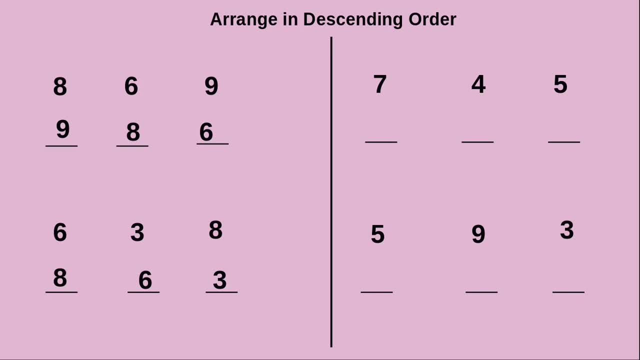 example, they have given 7, 4, 5, so which is the greatest number here? 7 is the greatest number, so we are going to write than 7 at first and then which one is greatest is 5 at last, which is remaining 4, so we are going to write as it is. 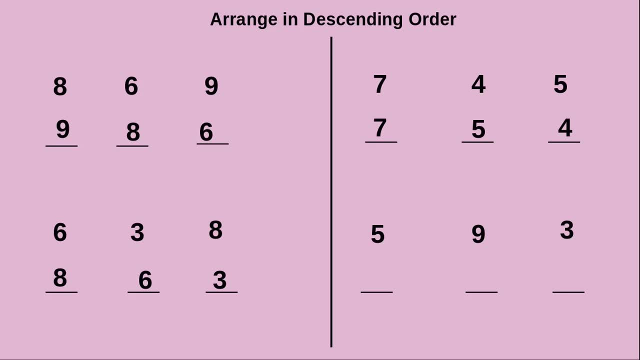 next, we are going to write as it is, so next, we are going to write as it is, so next we are going to. Next, we move to another example. they have given 5, 9, 3. which one is the greatest here? 9 is the greatest number, so we are going to write this first, after that, which one, 5 at last, which is 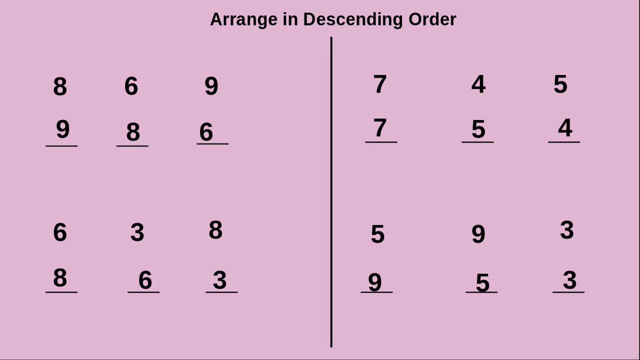 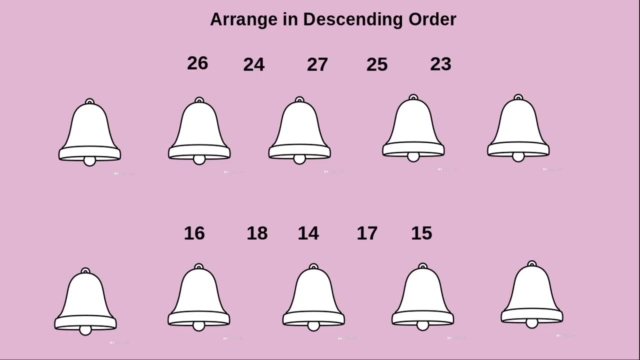 3. so now we are arrange these numbers in descending order. Next we will see some more example. now we are going to see how to arrange two digit numbers in descending order. so first we want to see the lost digit, that is, 6, 4, 7, 5, 3. so in this, which one is the greatest? 7 is the greatest, so 27 is. 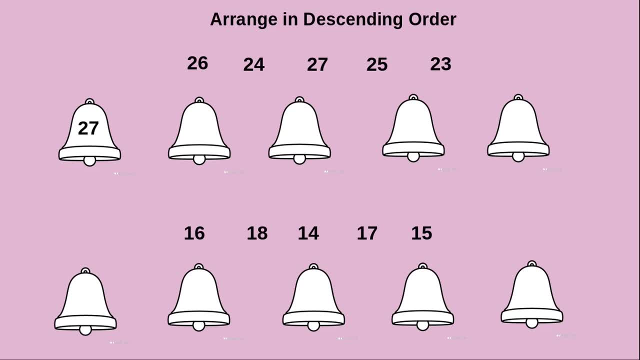 the greatest number. so we are going to write first 27, after that which one is greatest: 6. so 26 is the greatest number, after that 25, after that 24. at last, which is remaining 23, we are going to write it. Next. we will move to the another example they have given: 16, 18, 14, 17. 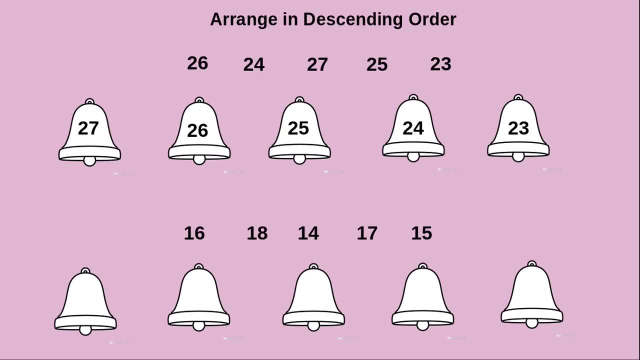 following 15. so which one is the greatest number here, any guess? yes, you are correct. so 18 is the greatest number. so we are going to write: first 18, next which one is the greatest number is 17, next which one 16, next which one it's 15, next which one it's 14. so now we all know how to arrange this number. 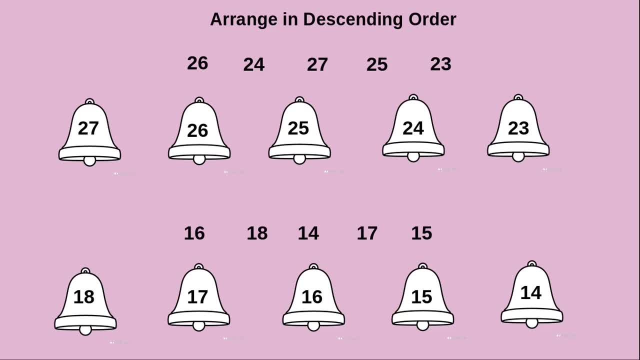 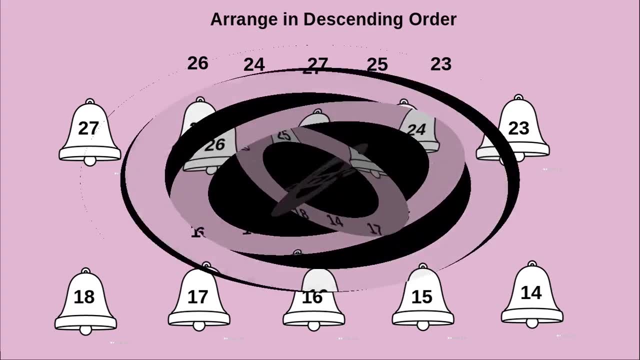 in descending order. okay, children, i think you all learn how to arrange the number in ascending order. in descending order. i hope you understand this concept. thanks for watching.